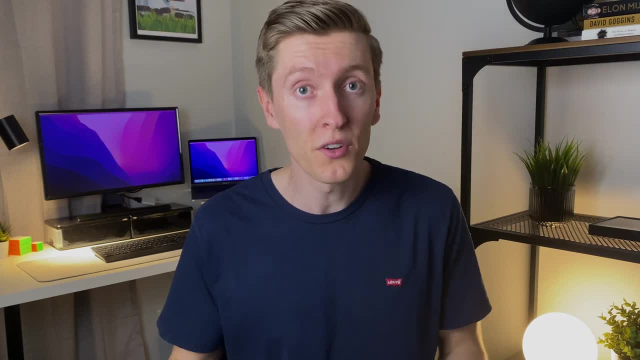 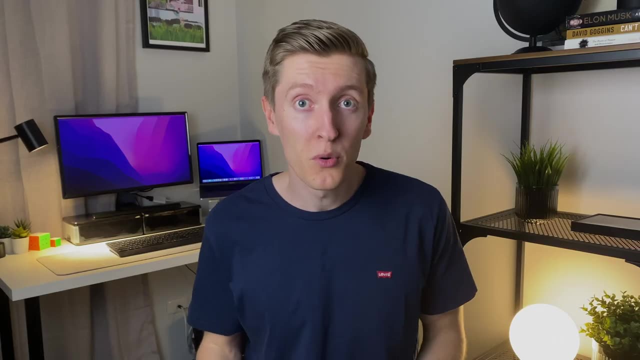 and started working at a mid-sized engineering firm, But what you definitely won't know is that during my job hunt, I did something I've never done before, and what I did was create a structural engineering portfolio. For those of you that don't know what a portfolio is: 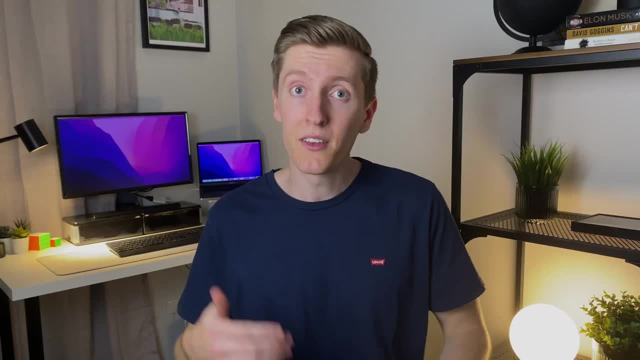 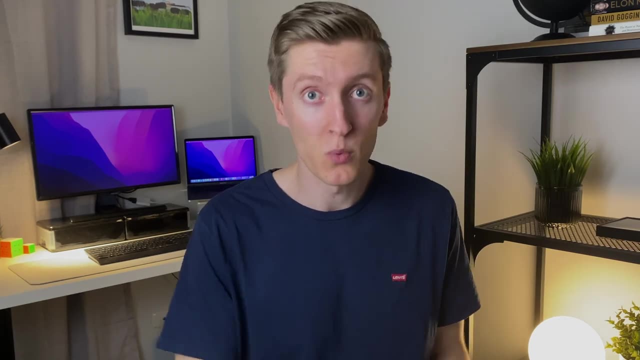 it's basically a short booklet that showcases your past work, and the idea is that the reader can get a better understanding of the quality and the type of work that you produce by actually taking a look at some of your past work. People in the film and television industry have been 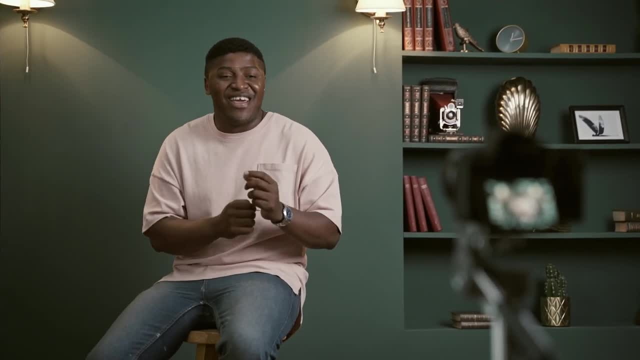 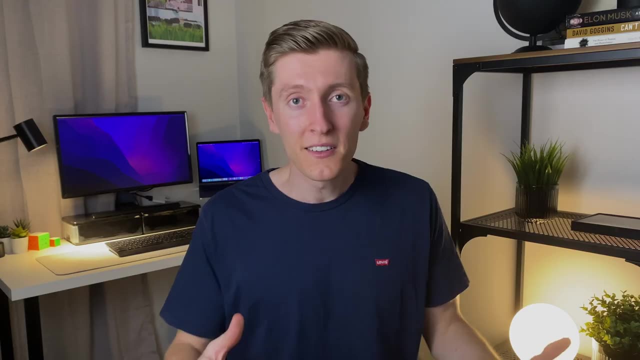 doing this for years through creating things like self-tapes and getting headshots taken, and now, in more recent times, this same idea has trickled into fields like web design and journalism, and now engineering. Currently, engineering fields like software- electrical and mechanical- are pretty used to the idea of creating a portfolio, But as far as I know, 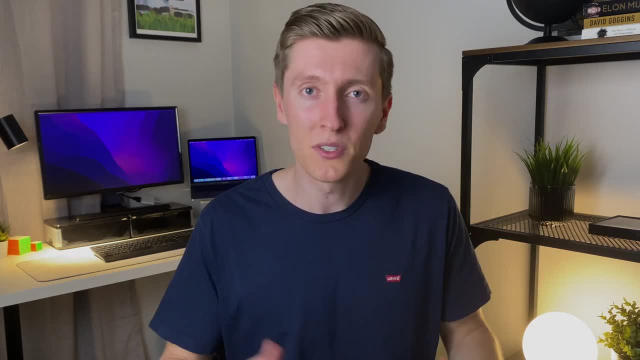 this same idea hasn't become a stock standard practice throughout the civil and structural engineering fields, So if you're interested in learning more about how to create a portfolio, please subscribe to my YouTube channel and hit the bell icon, so you don't miss out on any future videos. 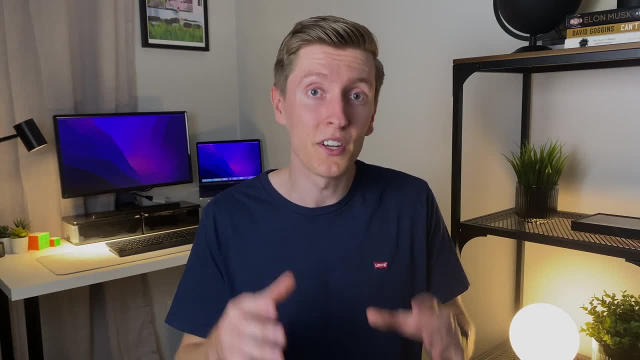 So if you're interested in learning more about how to create a portfolio, please subscribe to my YouTube channel and hit the bell icon so you don't miss out on any future videos. So in this video, I'm going to share what I learned from making a structural engineering portfolio. 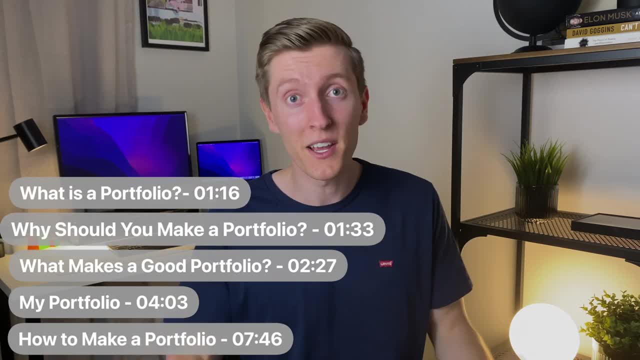 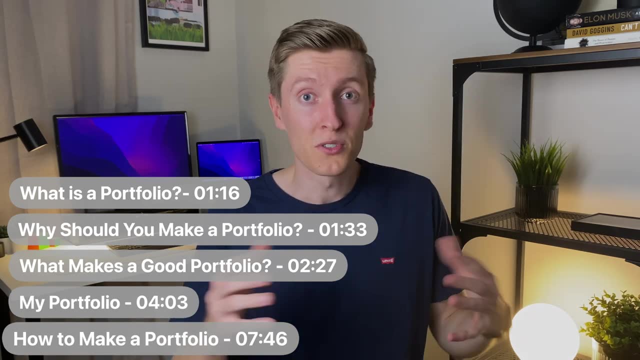 I'll go into more detail on what a portfolio is and why I think you should make one. what qualities make a good portfolio? I'm going to take you through mine and then I'm going to show you the full process of making a portfolio from scratch with a free. 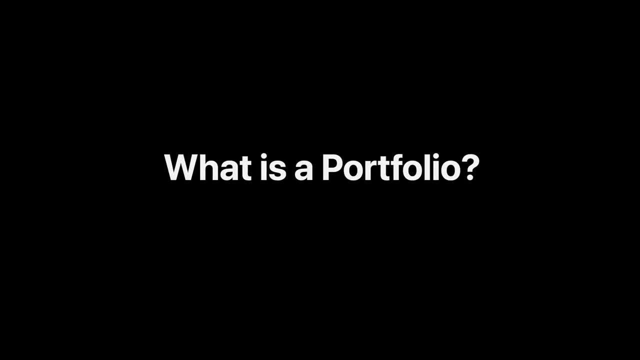 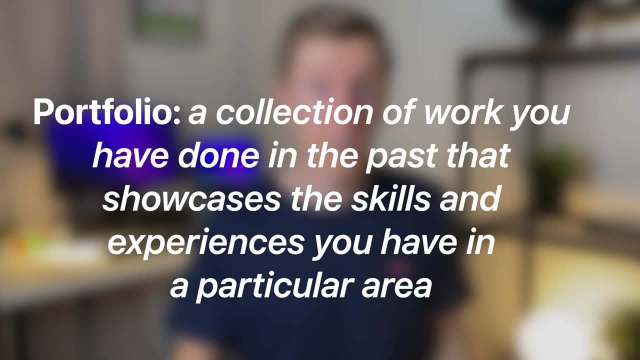 template at the end. Okay, so just to make sure that we're all on the same page. a portfolio is a collection of work you've done in the past that showcases the skills and experiences that you have in a particular area, And what a portfolio actually looks like is just a couple of. 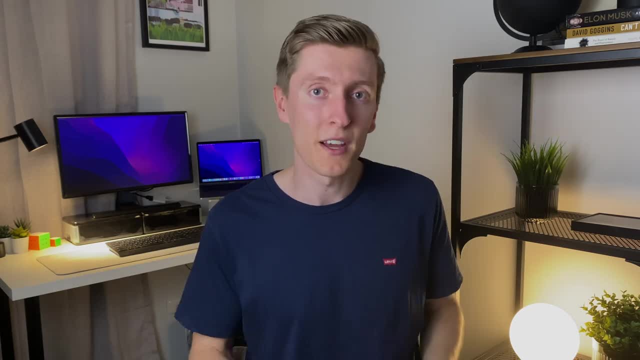 pages with images and explanatory text that gets attached to the back of your resume. All right, so now? why should you go through the effort and actually make a portfolio? Well, in my opinion, there's three main reasons you should. Number one is that it will differentiate. 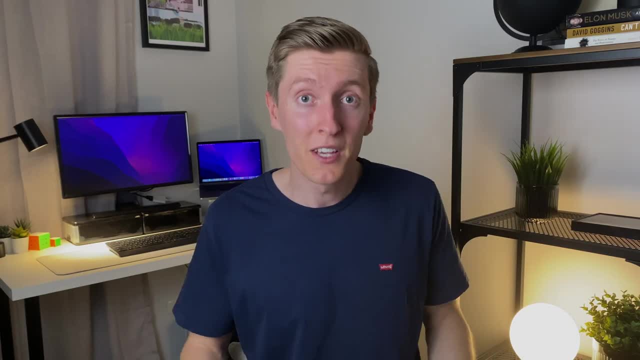 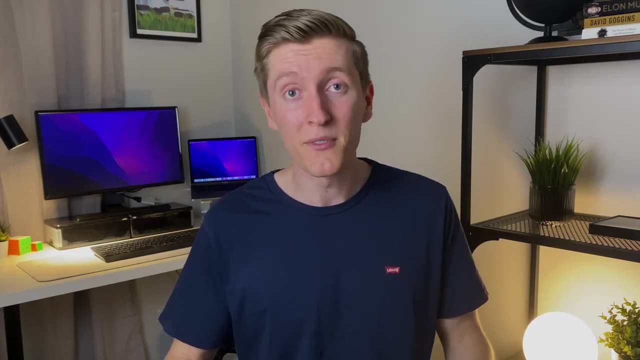 you from other candidates. Majority of people, when applying to new jobs, are only going to include a resume and perhaps a cover letter if it's required, But by also including a portfolio straight away, you're giving the recruiter a reason to progress your application. 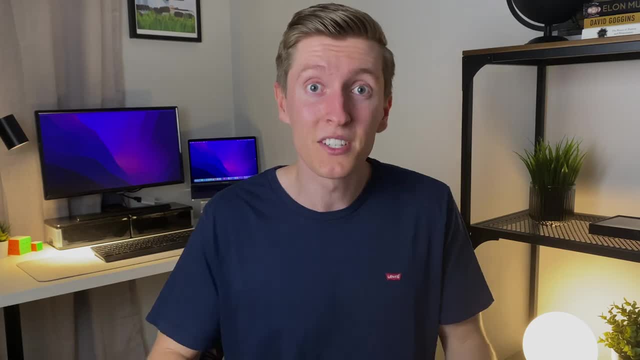 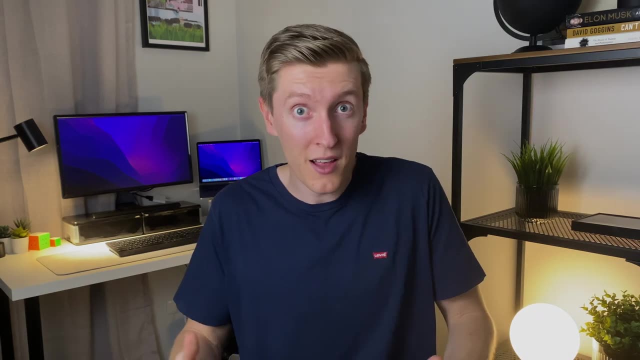 because you've gone the extra mile and don't blend in with all the other applications that all look the same. Number two is that portfolios provide context. A good portfolio easily allows the reader to visualize the projects you've worked on and quickly comprehend the level of skill you have. 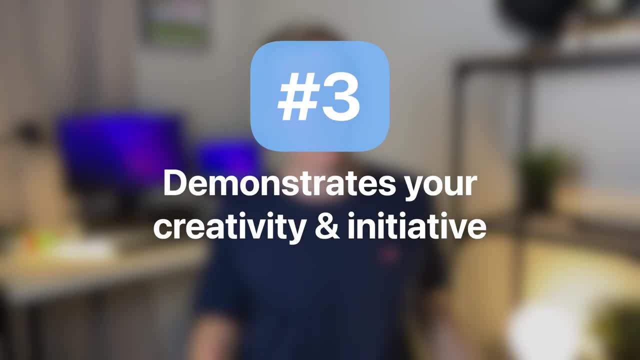 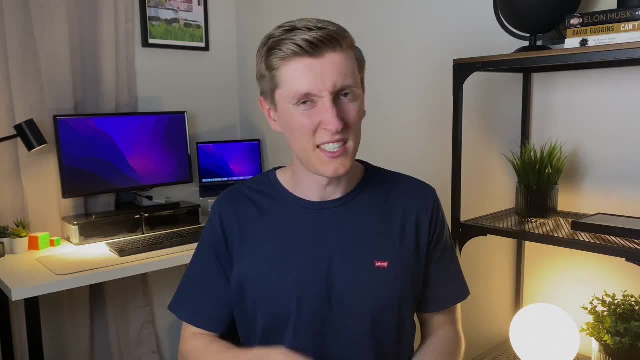 without tediously having to read through your resume. And reason number three is that a portfolio demonstrates your creativity and initiative. Given that a portfolio is not currently a requirement for job applications in the civil engineering related disciplines, by actually providing a portfolio, you're showing the recruiter that you're someone who is proactive. 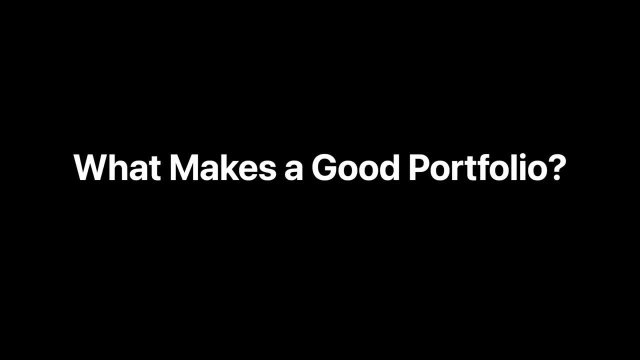 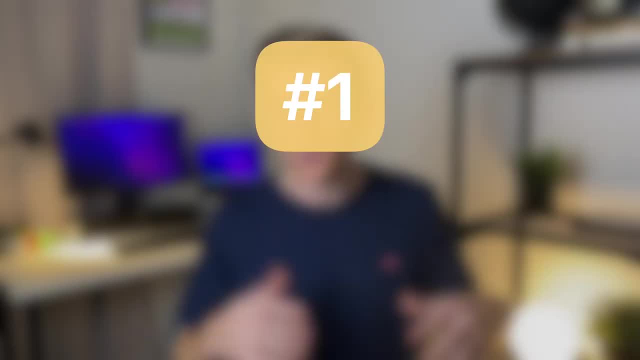 and that you're someone who is proud of their past projects. All right, I've convinced you that making a portfolio is worth your time. Let's talk about four important things to consider when making one that will really make it good. Okay, so first, a good. 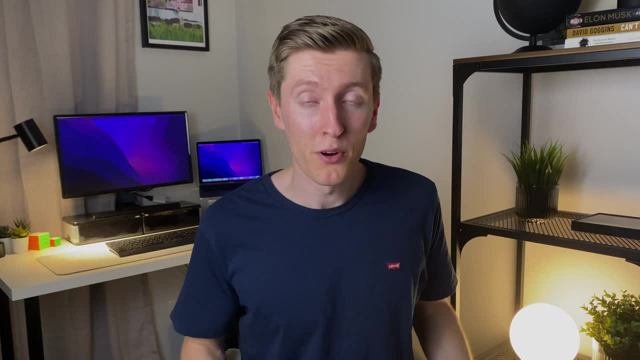 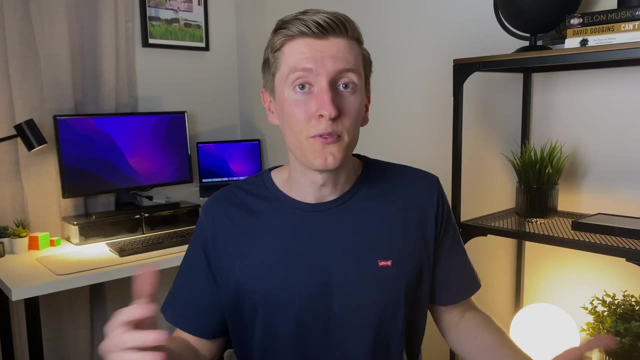 portfolio highlights a range of skills. This means that you should choose projects that have shown that you've worked with a variety of software programs, materials and structures. Second, include only relevant projects, So, for example, if you're applying to a structural engineering job. 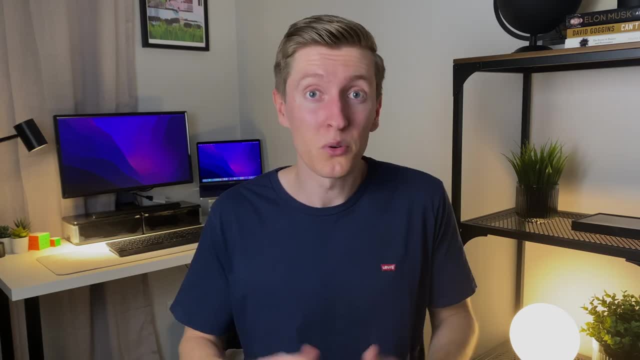 don't include projects from your civil or geotechnical engineering classes or internships. Third, include only your best work. So this means pick the best projects you've done during your classes or projects that you've worked on. So, for example, if you're applying to a structural 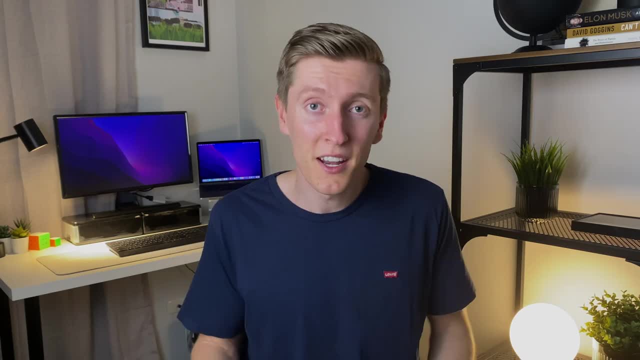 engineering job. don't include projects from your civil or geotechnical engineering classes or internships and showcase those projects. And if you're a student and you're thinking, well, none of the projects I've done so far are any good. I've got two options for you. 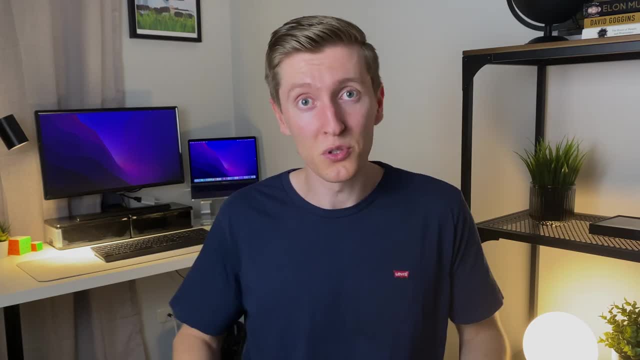 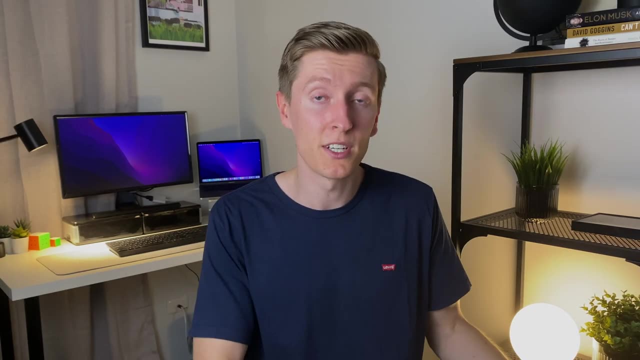 The first one only applies if you're a first or second year student and you've still got plenty of university projects ahead of you, But what I would recommend doing is changing your approach when it comes to completing your university projects. Right now, you're probably 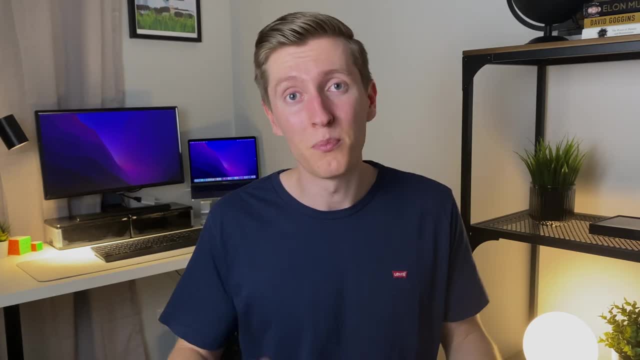 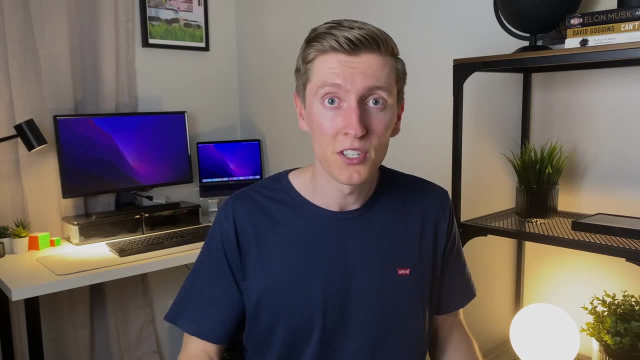 only completing your university projects to a quality that will allow you to pass the course, and that's why you wouldn't want to showcase them on your portfolio. So what you need to do is change your approach and start completing your university projects to a quality that will make them a portfolio worthy project, because now you're. 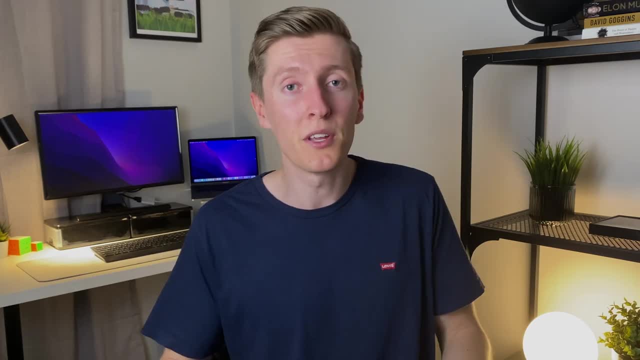 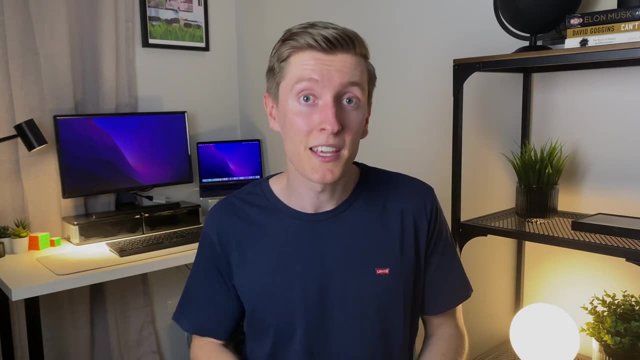 not only completing the projects to pass a course, but you're also completing these projects to help you land a job. Okay, and the second option you can do, regardless of where you are in your university journey and what it is, is making personal projects. For example, you could try and design. 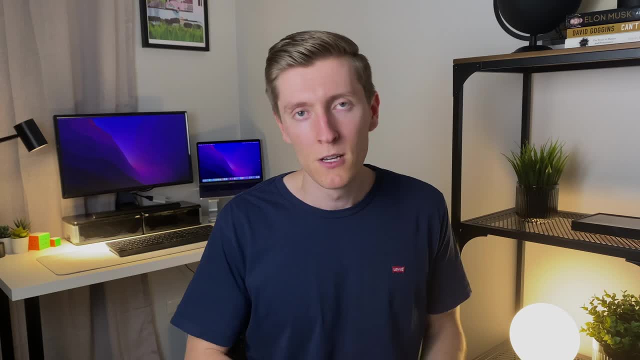 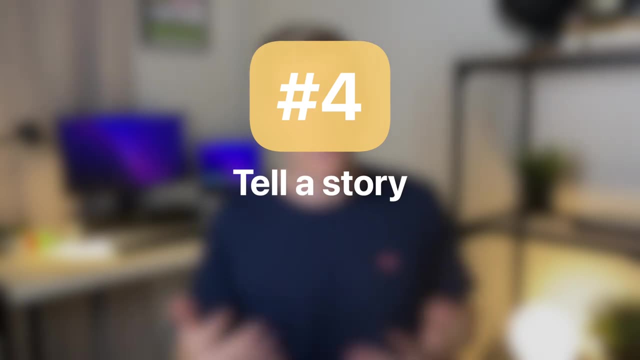 a simple steel frame structure, or maybe even just a concrete slab With personal projects. it's really up to you what you want to do, So just pick something and give it a go. All right. and the fourth and final thing that a good portfolio does is tell a story. Make sure. 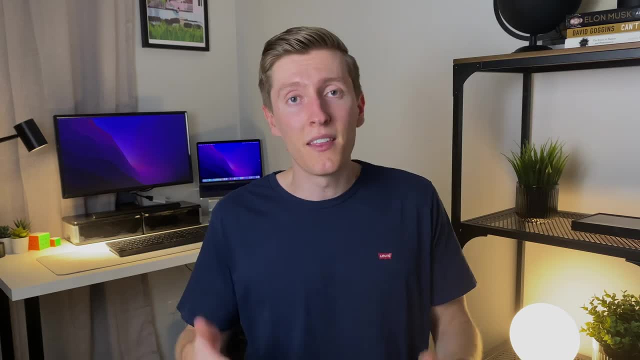 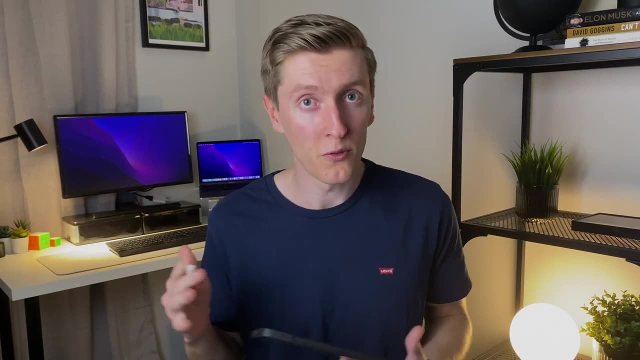 that your portfolio explains what you had to do, how you did it and then, where appropriate, what the result was. Okay, so now I'm going to take you through my portfolio and then I'm going to erase it completely and show you how to build a portfolio from scratch. 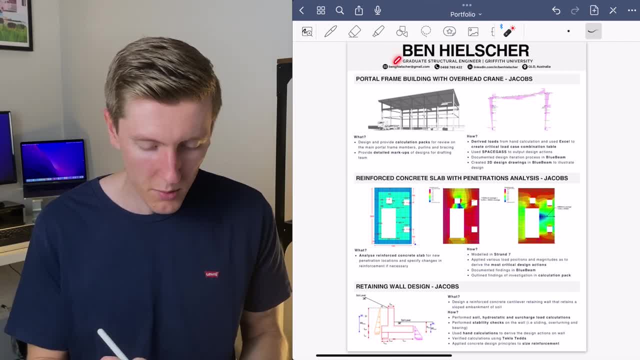 All right. so, starting off the top, I have my name, the type of role I'm applying for and also the university I graduated from. Underneath this, I have my contact info. Here I included my email, my phone number, a link to my LinkedIn profile and also the state and country. 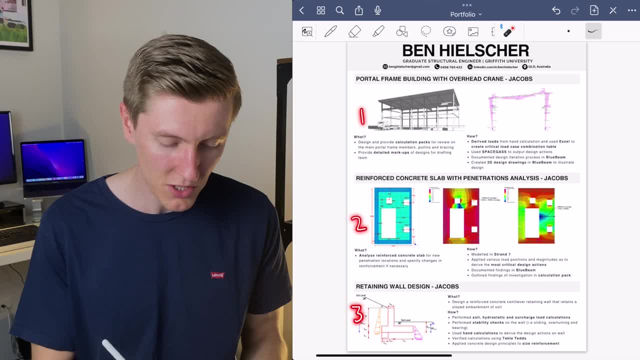 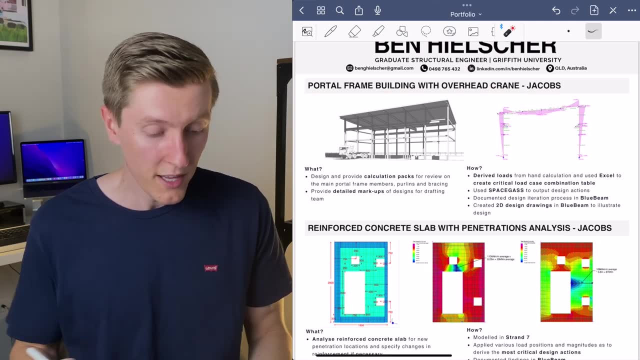 I live in Below the title block. I've broken the page up into three sections where I showcase each project. Up the top is my first project, which is a portal frame building with an overhead crane that I did while I was at Jacobs. On the left I have a screenshot of an architectural drawing. 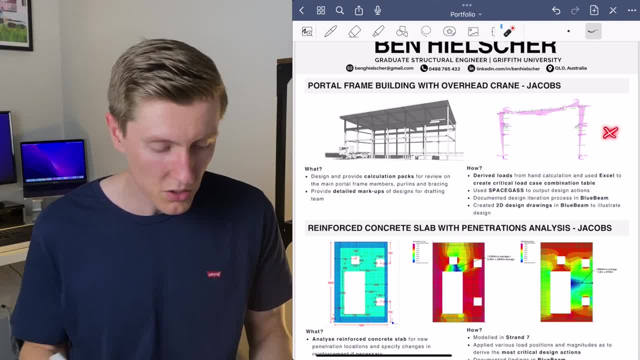 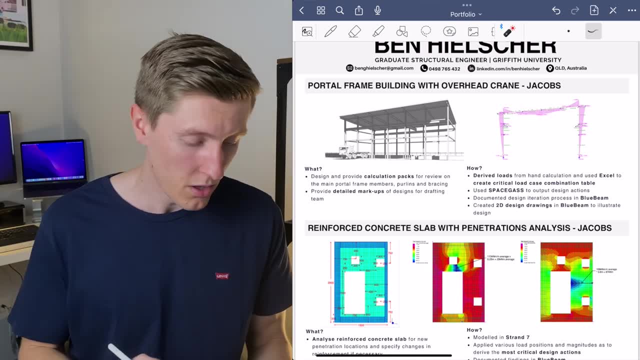 of the building so it's easier to visualize the project, And on the right I have a screenshot of a portal frame with a bending moment diagram drawn on it, and it's taken from the structural analysis program Space Gas. In the text section below I have two headings: what and how. 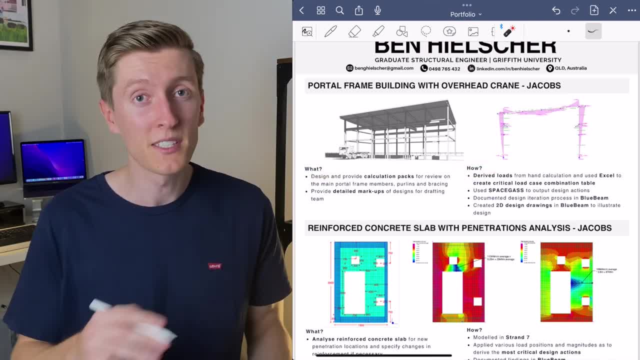 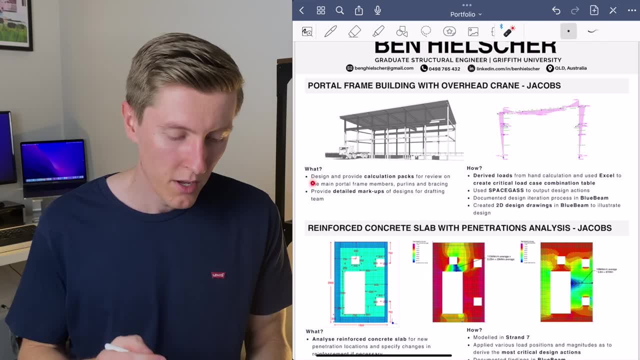 and the idea here is that under the what heading I would show what responsibilities I had and then under the how heading I would show how I executed those responsibilities. For example, in the what section of this project I wrote: design and provide calculation packs for review. 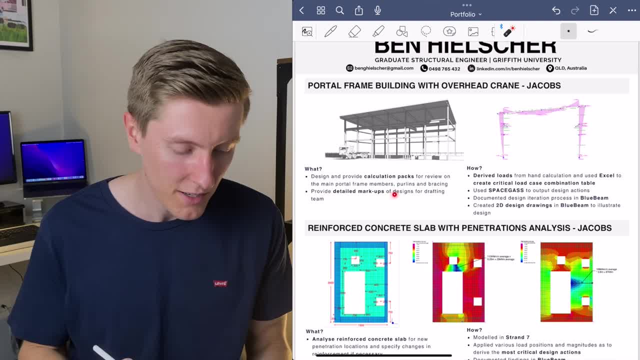 on the main portal. frame members Perlins and Bracing and provide detailed markups of designs for drafting team. Then in the how section I wrote: derive loads from hand calculation and used Excel to create critical load case combination table. use Space Gas to output design actions. 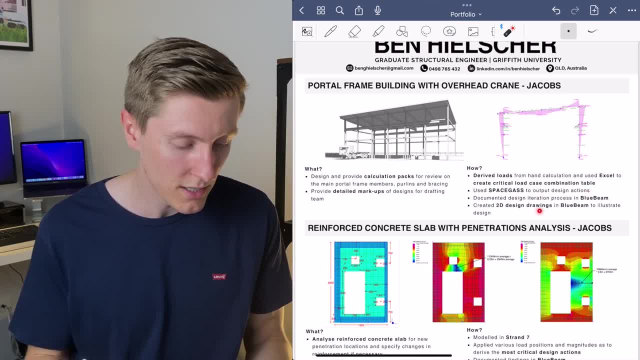 document a design iteration process in Bluebeam and created 2D design drawings in Bluebeam to illustrate design. One thing I do want to point out here that you may have noticed is that throughout this text I've bolded any word that highlights a technical. 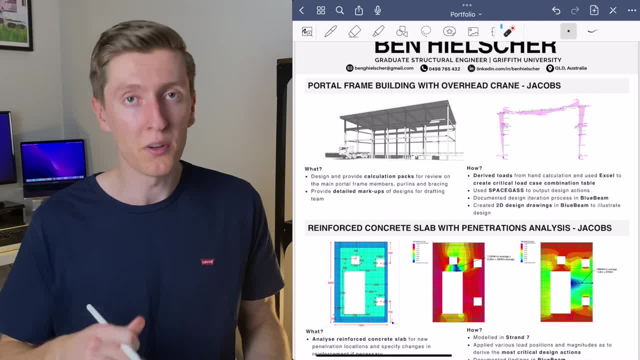 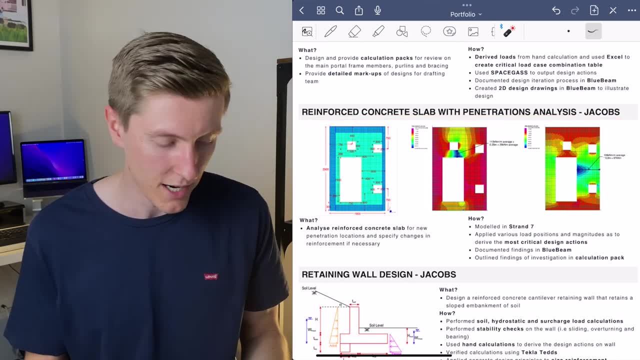 skill that someone in my role might have, so that it's easy for the reader to pick up on. Okay, and moving on to the second project in my portfolio, which is a reinforced concrete slab analysis that I also did while I was at Jacobs. Notice that, again, I'm following the same what? 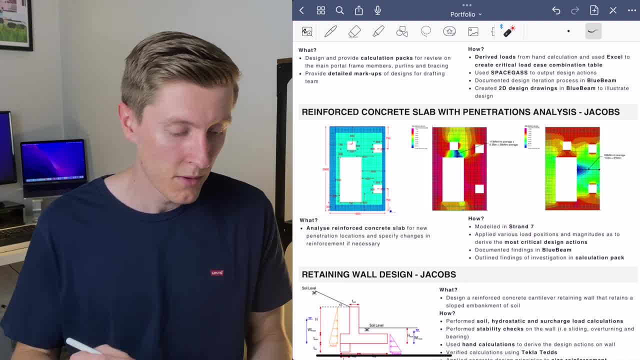 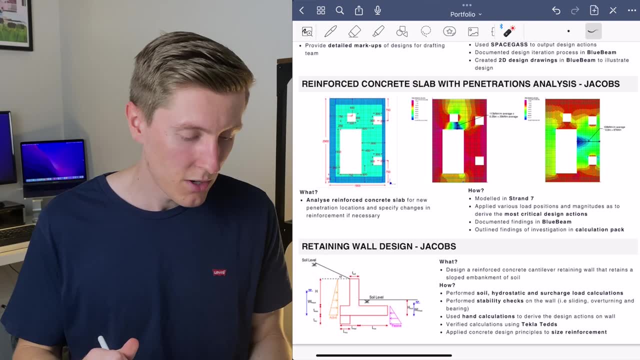 and how format, and that the pictures I'm showing are from a different software program and that in this project I've shown something to do with concrete rather than steel, to try and show the reader that I'm confident with this material too. Okay, and the next project in my portfolio. 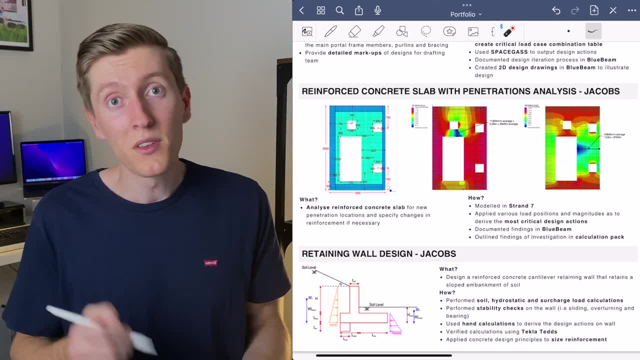 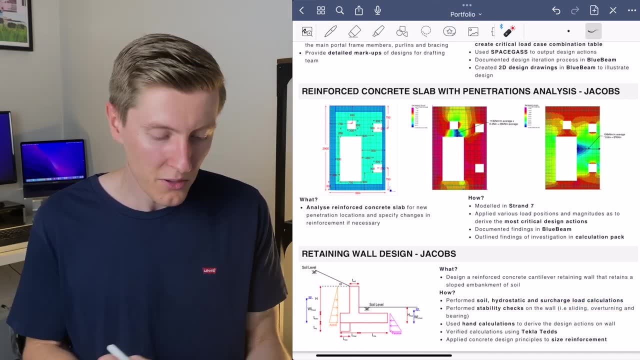 was another project I did at Jacobs and this one's a retaining wall design. With this particular project I've got loads and checks we need to do when designing earth retaining structures and I think, with the little bit of text that I have and the diagram I've drawn, 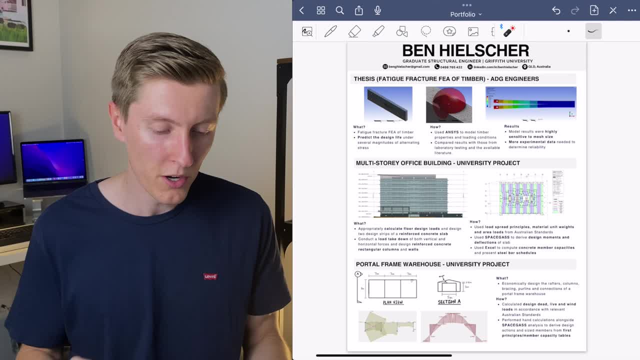 I've done that well enough. Okay, and over the page I've got three more projects, and the one up the top is from my thesis that I completed during my time at ADG, and the two down the bottom are ones that I completed while at university. 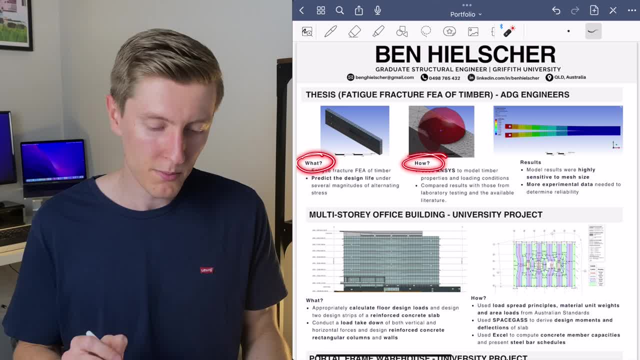 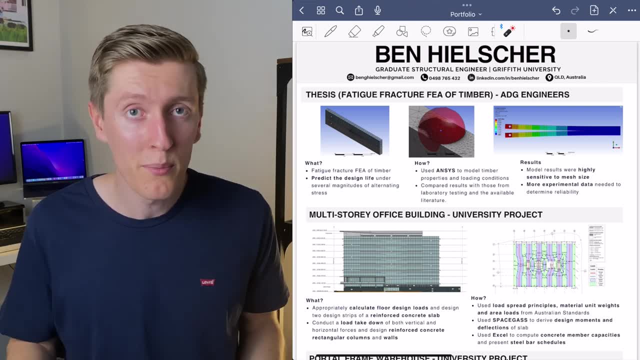 Starting with my thesis up the top. I decided to separate the headings for this project out into three sections because for this particular project I actually had tangible results that I could share And similar to what I've done for my projects on the first page. 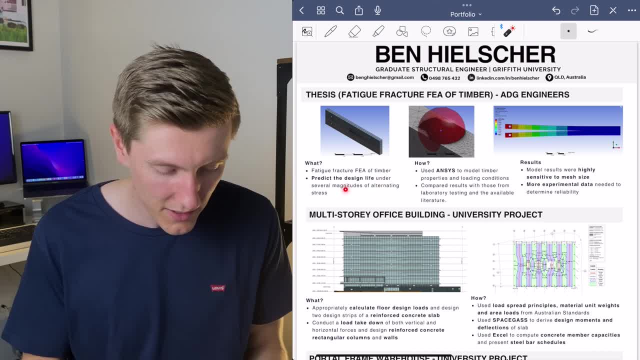 I've said what I had to do, which in this case was predict the design life under several magnitudes of alternating stress, how I did it, which was used- ancestor model timber- and compared results with laboratory testing and literature and finally, what the results were. 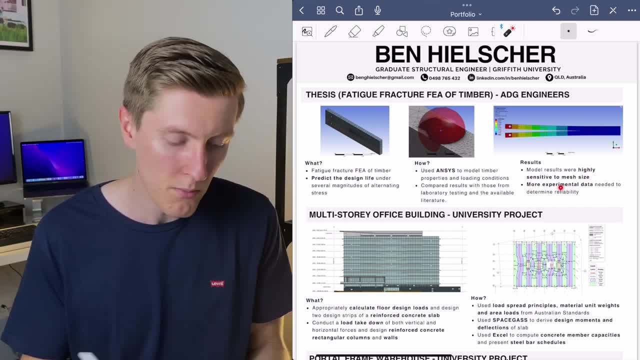 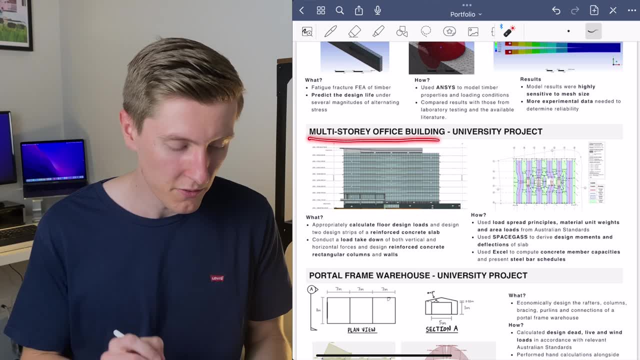 which was that the model was highly sensitive to mesh size and that more experimental data was needed to determine the reliability. Okay, and moving on to my first university project, which I've labeled multi-story office building, Here I've got a screenshot of what the building. 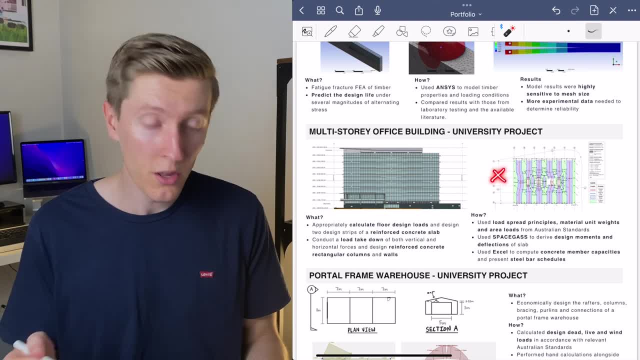 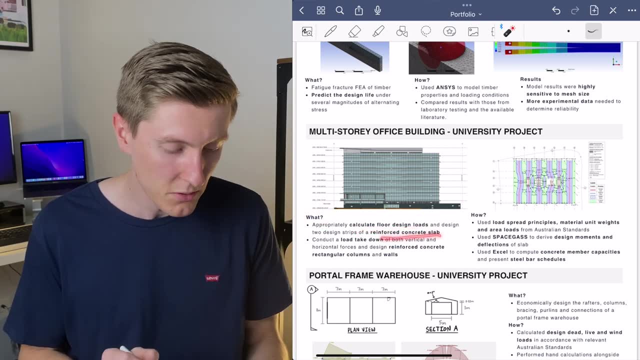 looked like on the left and then on the right. I've got a screenshot of a column in middle strip sketch that I did when doing this lab design. Again, I'm explaining exactly what I had to do on the left and I'm trying to bold as many technical skills that I had to use as 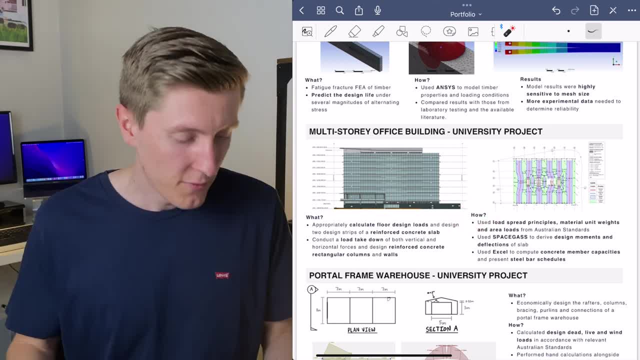 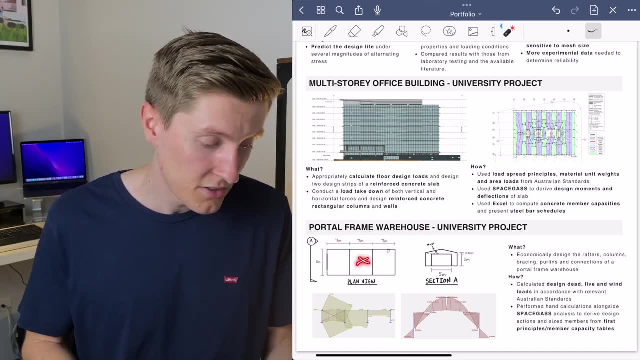 possible and then on the right, how I executed those tasks. Okay, and finally, the last project on my portfolio was a steel portal frame warehouse design that I did for a class at the end of second year. Here I've got some screenshots of some hand sketches that I drew of the geometry. 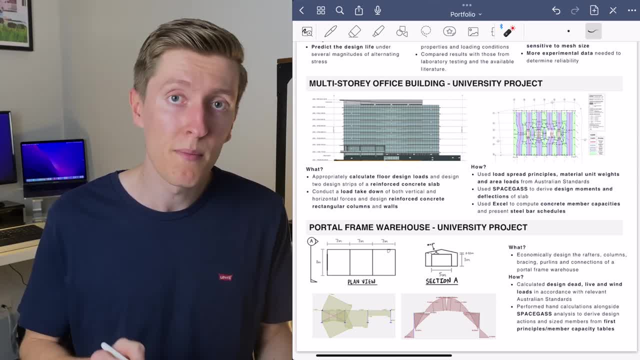 and also some from space gas that I used when designing the main portal frame members and also the bracing. In the what section of this project, I wrote that I had to economically design the rafters, columns, bracing and the structure of the building. And then I've got. 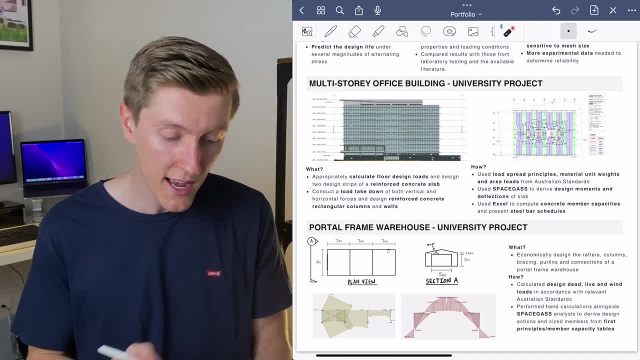 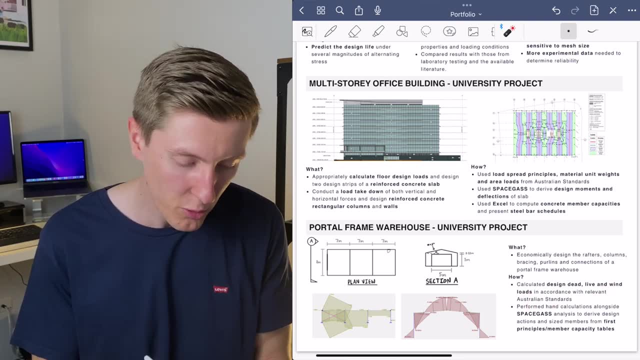 a screenshot of a portal frame warehouse design and then in the how section I wrote that I did this by calculating dead, live and wind loads in accordance with relevant Australian standards and by performing hand calculations alongside space gas analysis to derive design actions. 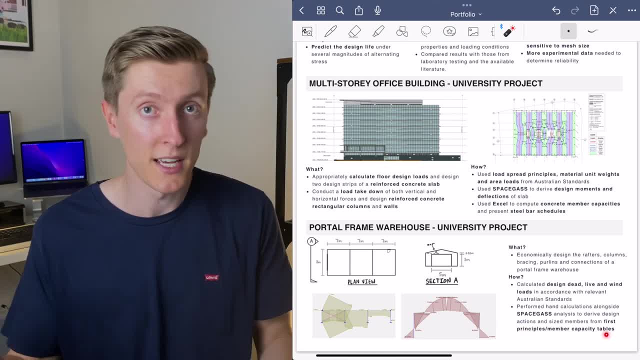 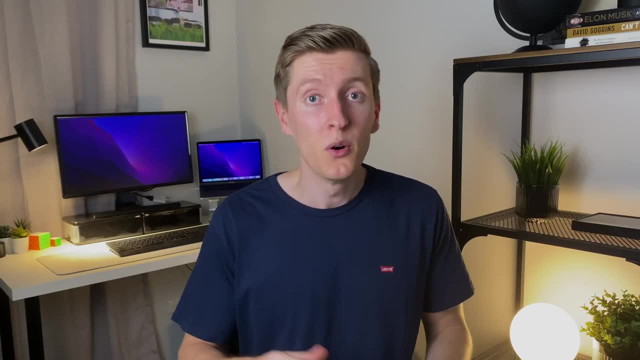 and that I sized members from. first principles: slash member capacity tables. Alright, now that I've shown you what my portfolio looks like, let me erase it completely and show you how you can build something similar from scratch. Also, if you like the way my portfolio looks, you can download my free Canva template through. 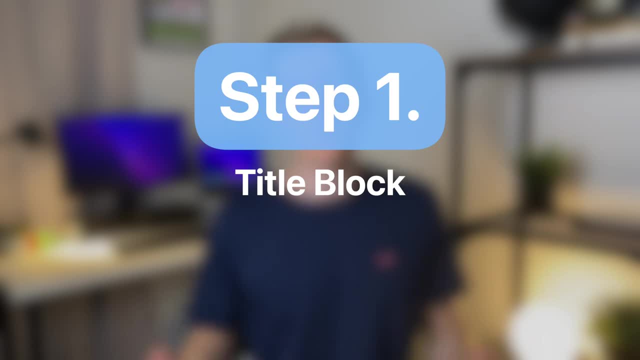 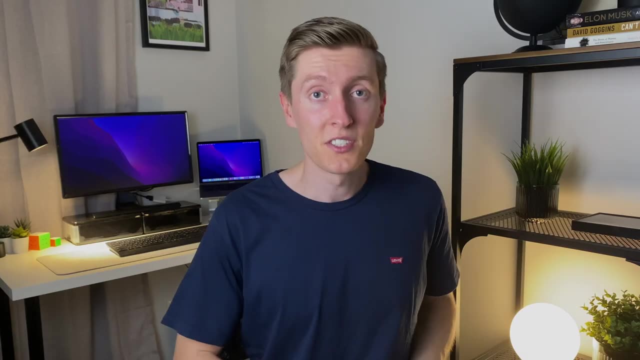 the link in the description. Okay, so first up, let's begin by doing the title block. Here you need to add your name, title, university and contact details. Next, make a list of all the projects you've done during university and any internships and select the ones you want. 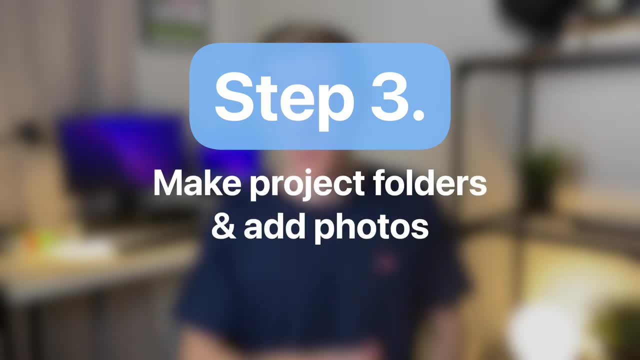 to include From here. you should make a folder on your computer for each project and put all the photos or screenshots you have from those projects in these folders. After this you should decide on what order you want to put your projects on your portfolio.